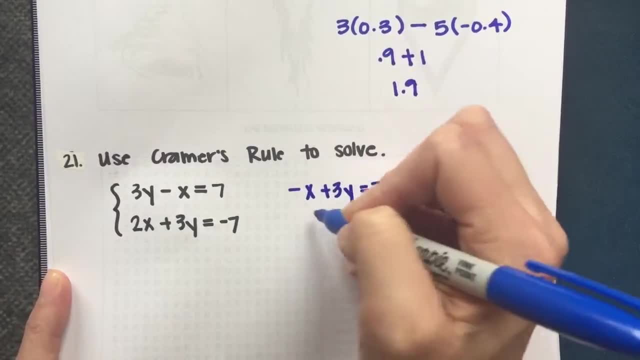 So negative x plus 3y equals 7, and then 2x plus 3y equals negative 7. 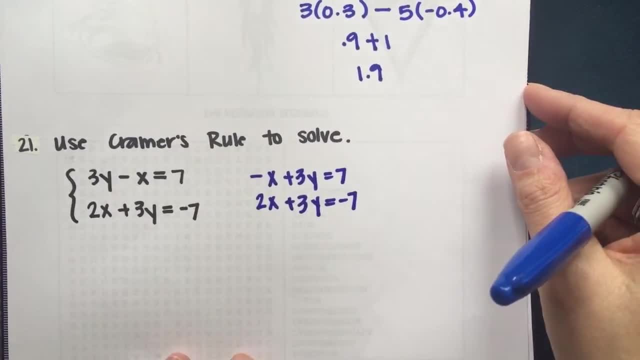 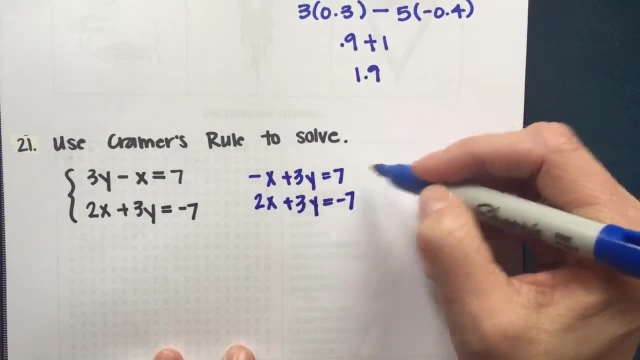 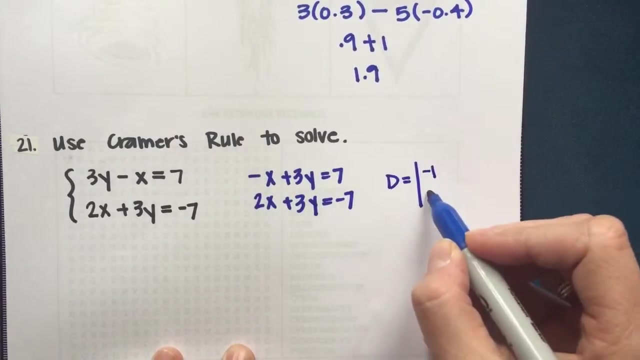 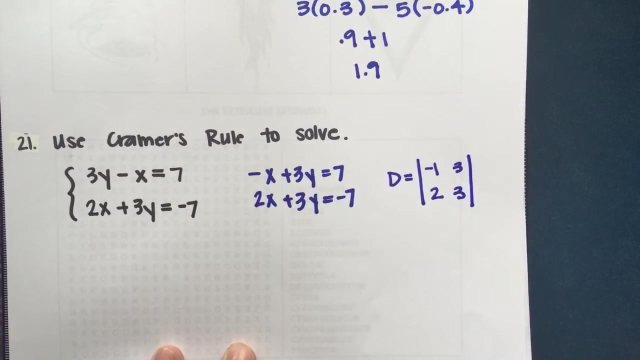 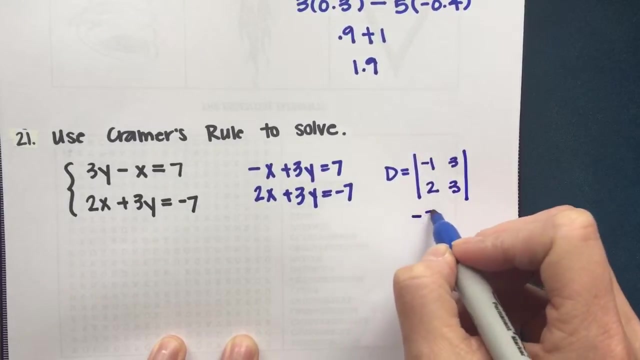 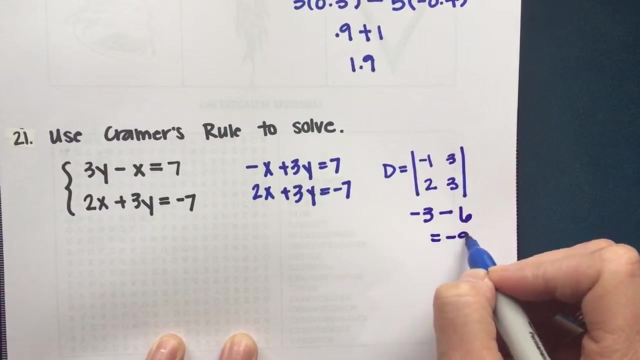 So I'm going to write the coefficient matrix first. That's my capital D that's going to go on the bottom for Kramer's rule. The coefficients are the numbers in front of these variables. So we're going to keep them in the order that they're in right now. D is the determinant. The determinant of the coefficient there is negative 1, 2, and then the y column, 3, 3. So we have a 2x2 matrix now that I'm going to do like I did in the previous problem. Multiply the main diagonal, negative 1 times 3 is negative 3, minus, multiply the second diagonal, 3 times 2 is 6, and that is negative 9. 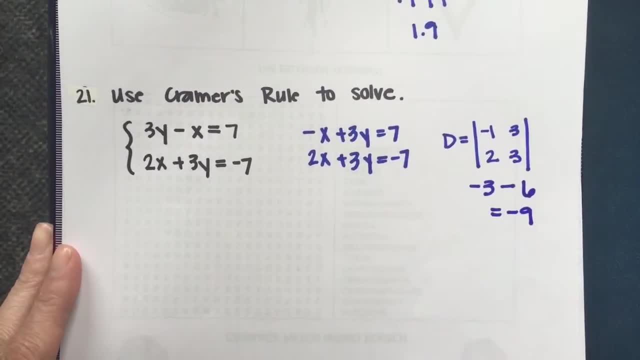 So the determinant for that is negative 9. Now we need to actually solve for x. So I'm going to set up for x. 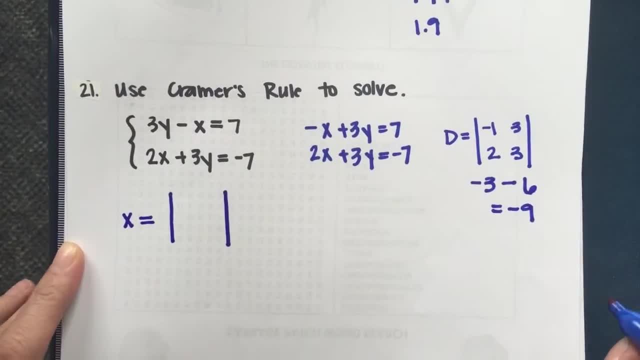 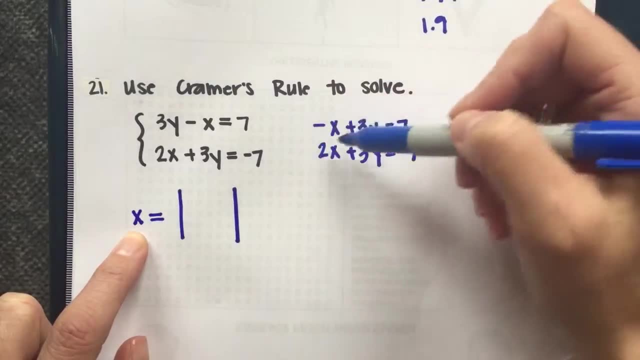 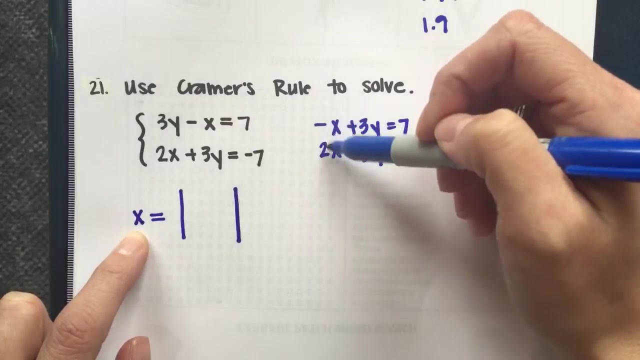 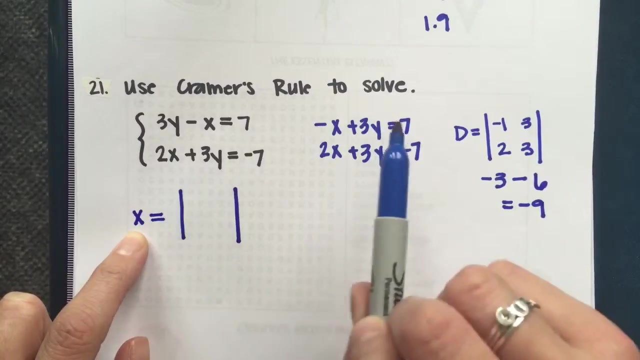 It's the determinant of a new 2x2 matrix. And in that new 2x2 matrix, I'm going to, if I'm solving for x, I'm going to replace the x column. So I'm going to not use the x coefficients, but instead of those, I'm going to put in the constants. So since x is on the left, the x coefficients went on the left-hand side, I'm going to not use those. Instead, I'm going to use the x. use the constants, 7, negative 7. 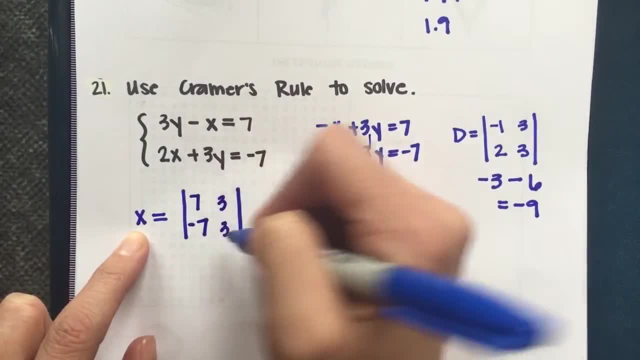 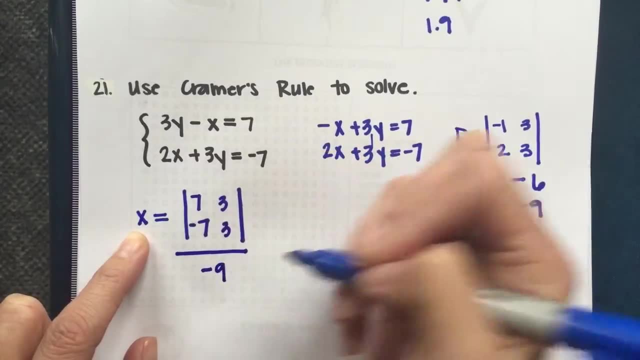 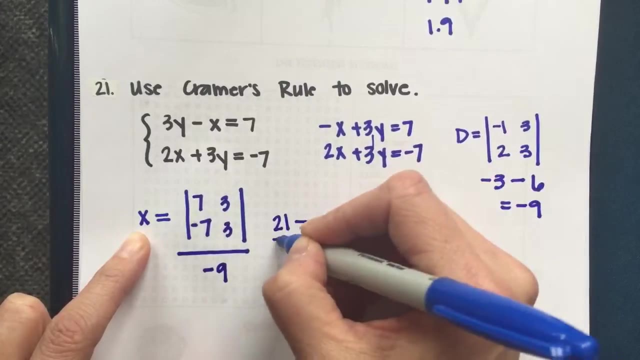 You keep y in there, so we're going to keep the 3, 3. And then it's over d, which was negative 9. So we get 21 minus negative 21 over negative 9, which is 42 over negative 9. 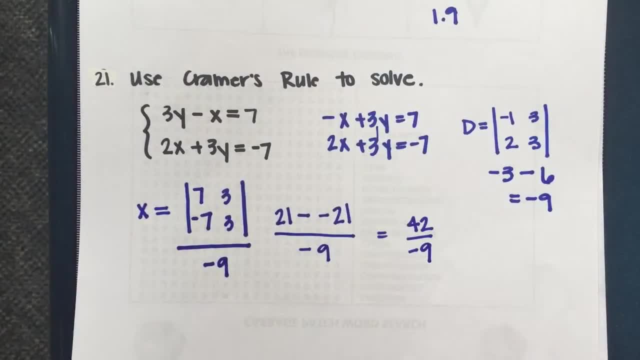 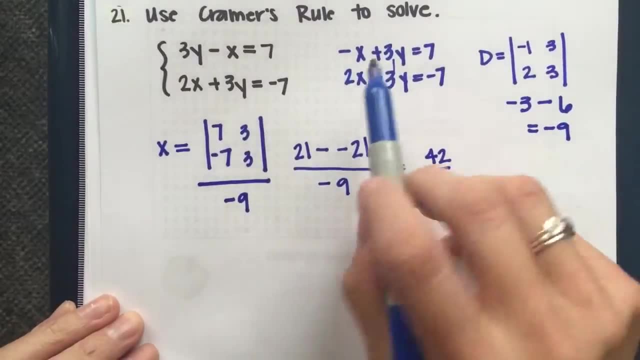 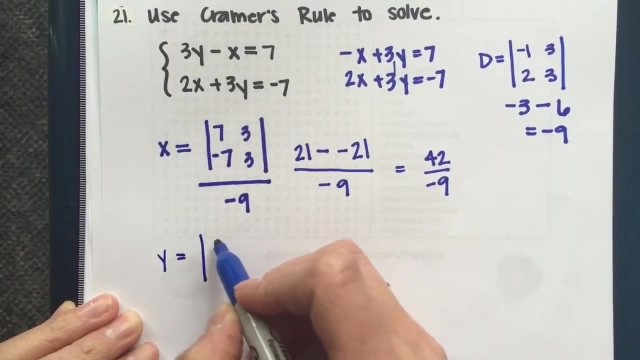 We have to solve for y also. So when we solve for y, I'm going to replace the y column with the constants. So I'm going to keep the coefficients from x, negative 1, 2.